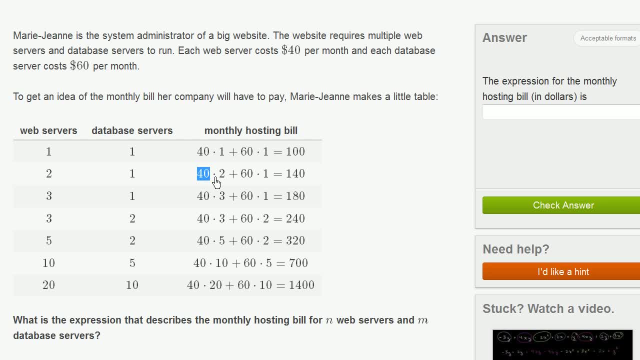 she has two web servers and one database server. So here she's multiplying 40 times 2, because that's how many web servers she has. so she's going to have to pay $80 a month for the web servers and still $60 per month for the one database server. 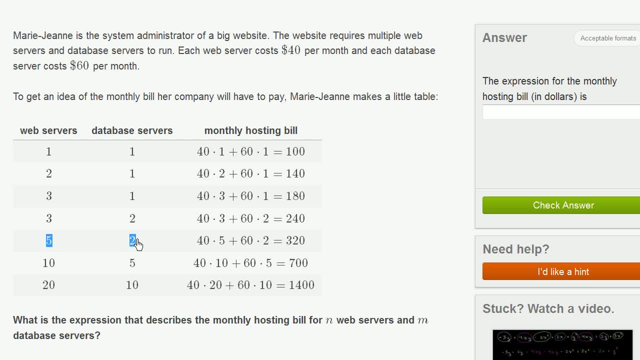 Let's skip to one that's more interesting. So here she has five web servers and two database servers. So she pays $40 per month for each of the five web servers and she pays $60 a month for each of the two database. 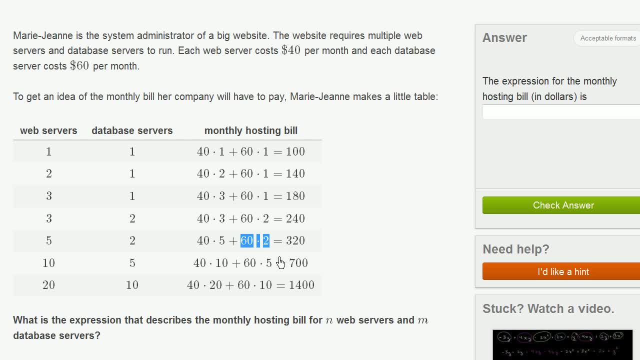 servers. So if you wanted to write an expression that describes the monthly hosting bill for n web servers and m database servers, well, you see here this pattern. She pays $40 per month for every web server that she has. So if she has n web servers, she's. 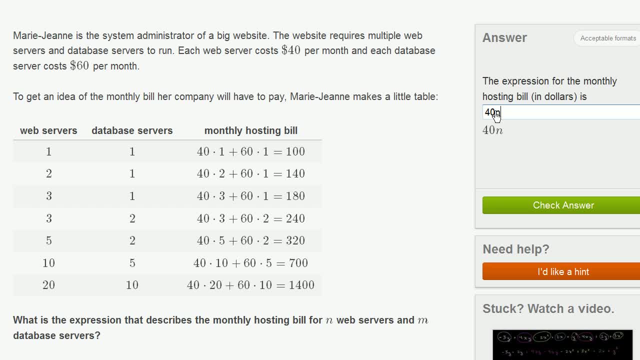 going to have to pay $40 per month per server times n servers. And then she's paying $60 a month per database server. So if she has m database servers she's going to have to pay $60 per month per server times the number of servers. 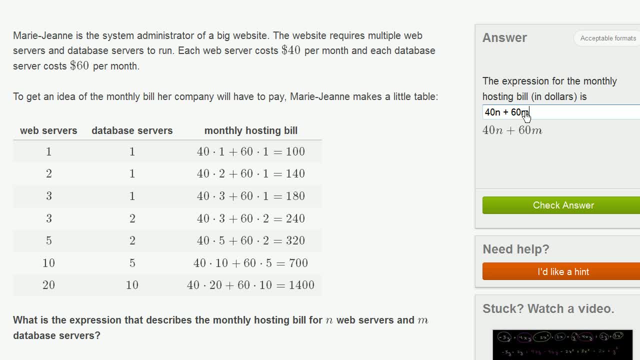 So this right over here is the expression for the monthly hosting billing cost And you could see that right over here. If you view this as n- the number of web servers- and this as m, you see that when n is 20 and m is 10,. 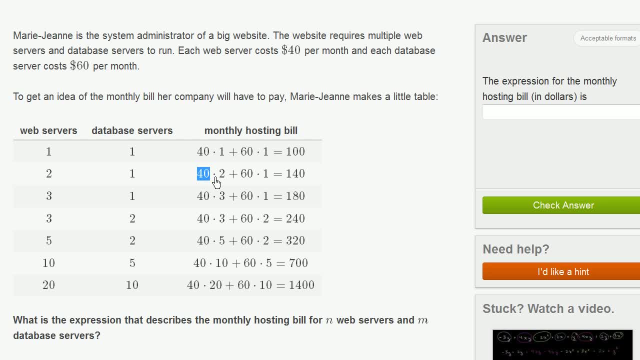 she has two web servers and one database server. So here she's multiplying 40 times 2, because that's how many web servers she has. so she's going to have to pay $80 a month for the web servers and still $60 per month for the one database server. 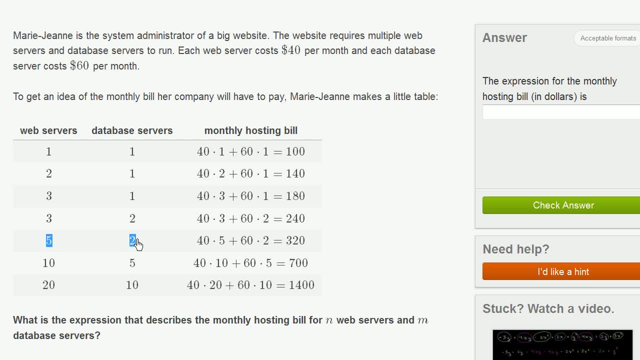 Let's skip to one that's more interesting. So here she has five web servers and two database servers. So she pays $40 per month for each of the five web servers and she pays $60 a month for each of the two database. 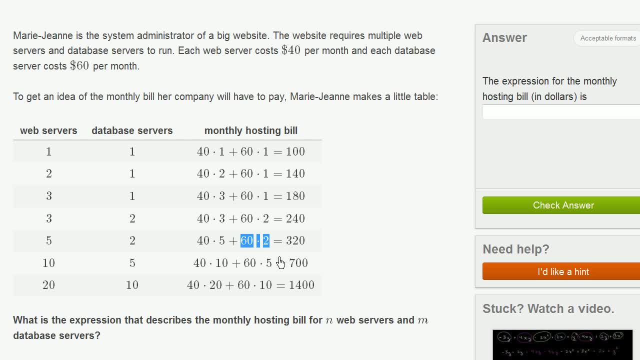 servers. So if you wanted to write an expression that describes the monthly hosting bill for n web servers and m database servers, well, you see here this pattern. She pays $40 per month for every web server that she has. So if she has n web servers, she's. 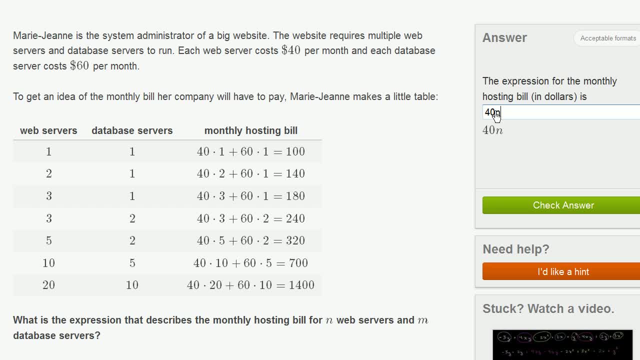 going to have to pay $40 per month per server times n servers. And then she's paying $60 a month per database server. So if she has m database servers she's going to have to pay $60 per month per server times the number of servers. 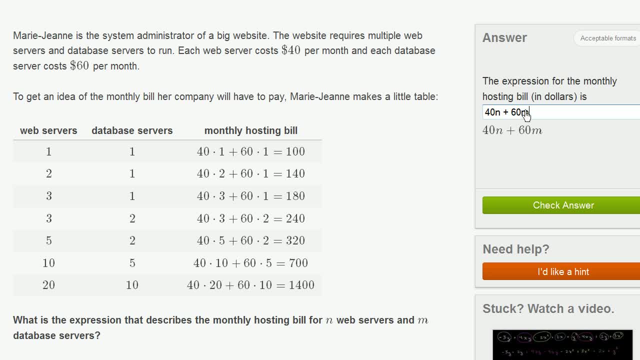 So this right over here is the expression for the monthly hosting billing cost And you could see that right over here. If you view this as n- the number of web servers- and this as m, you see that when n is 20 and m is 10,.